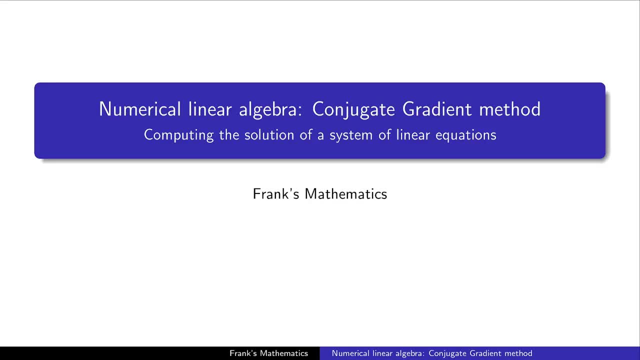 In this video I will talk about the conjugate graded method, which is a very famous method for computing the solution of a system of linear equations. Hi, my name is Frank and welcome on my channel. We will deal with the following system of linear equations which contains n variables. 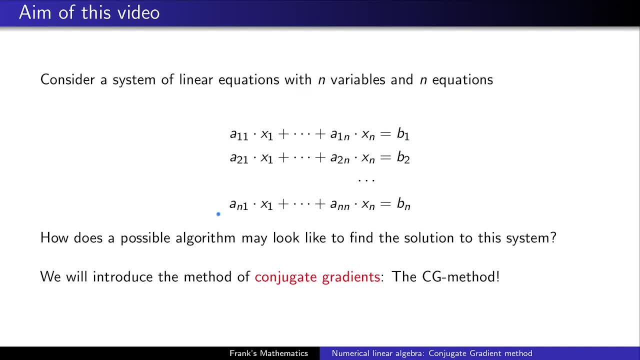 and n equations and they are coupled in the following form: And the question is: how does impossible algorithm may look like to find a solution to this system? And in the following I will introduce you to the method of conjugate gradients, or in short, the SIGIM method, which is a 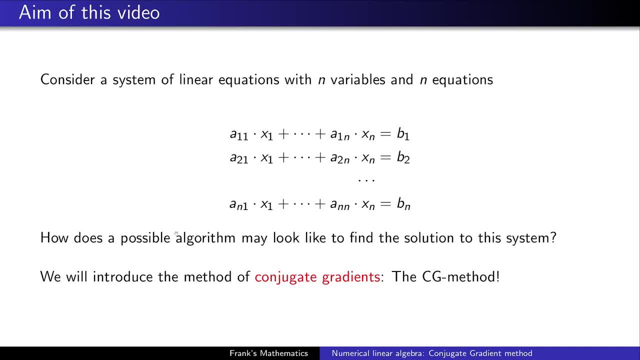 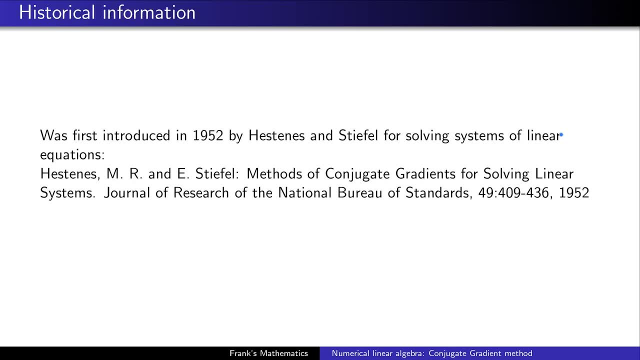 very famous method for solving such a system if the coefficients a satisfy a specific form. But we'll come to this later. Before we start with mathematics, we'll do some historical information. The method was first introduced in 1952 by Hestenes and Stiefel, So it's 70 years old. 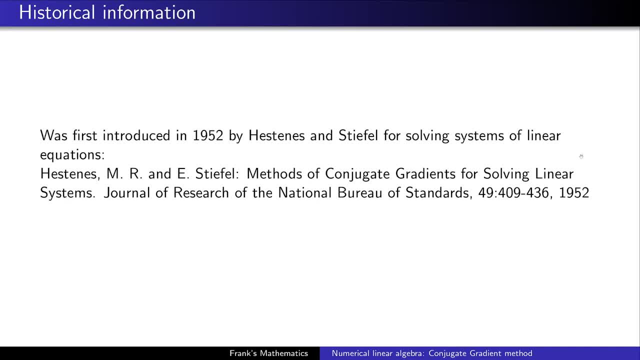 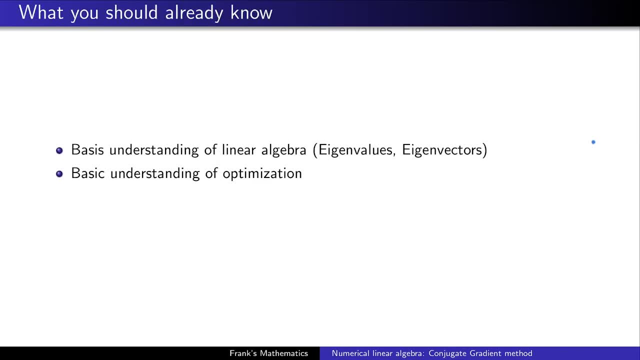 It's quite an old method, But it is a very super and a very efficient and very famous method. You should already know some stuff to understand this video. In particular, you should have a basic understanding of linear algebra. In fact, you should know about eigenvalues, eigenvectors. 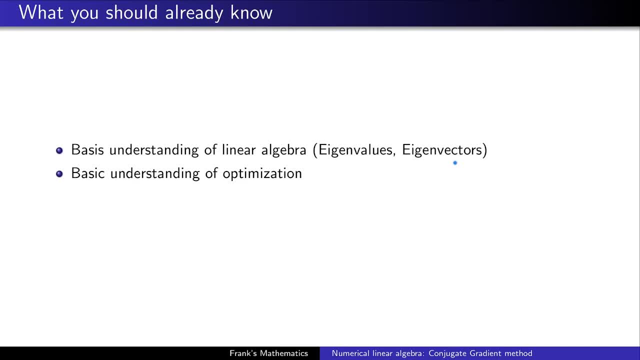 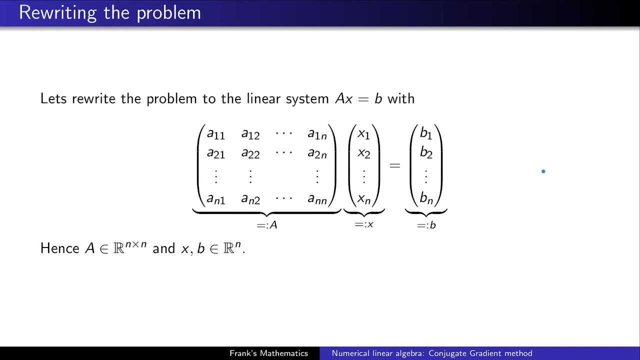 the eigenvalue decomposition, how to handle matrices, matrix vector multiplication and stuff like this, And it's good to have some basic understanding of optimization. Although it's not necessary to understand this video, I will introduce you to everything you will need Before we start. we will rewrite the problem to a linear system: xt equals b with some matrix a. 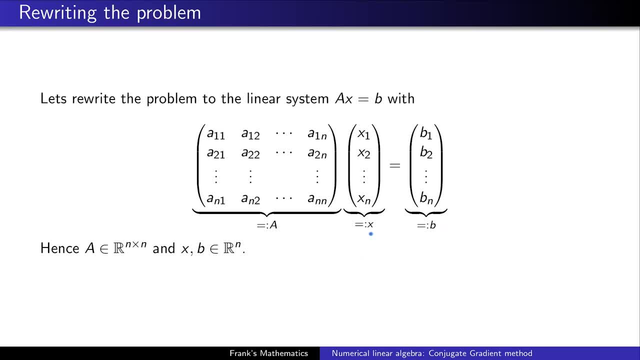 some right-hand value vector b and some unknown vector x which we are looking for. This is standard transformation. It's just matrix vector multiplication. Of course a is a real and times n matrix and x and b are the vectors in the space. are n. 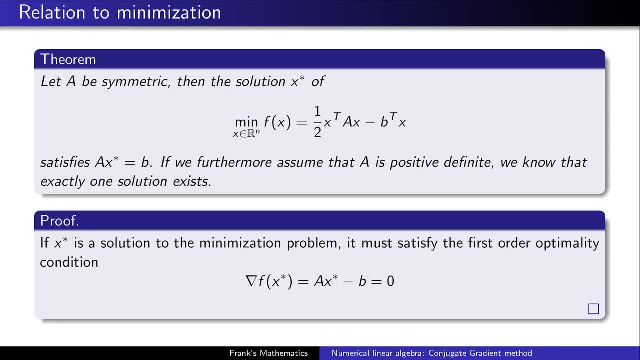 If you've watched a video of me, you probably know that I'm a huge fan of optimization, and rewriting problems into optimization form is usually a huge boost to understanding what's actually going on here, to understand the problem and probably to find a solution. So in our case here we are looking at the following function: 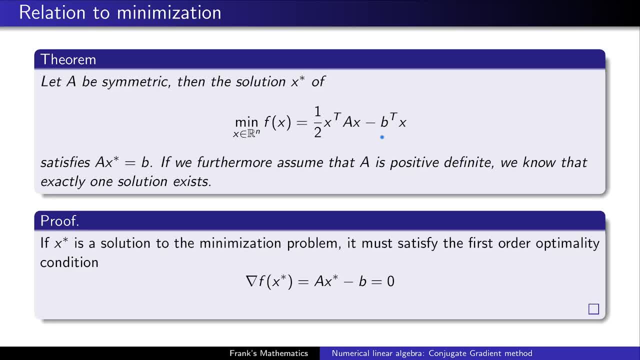 We want to minimize the following function: x transpose a, x minus b transpose x. And in the following we assume that a is a symmetric matrix. If we do so, we know that the solution of x star, of this optimization problem, satisfy a. x star equals b. 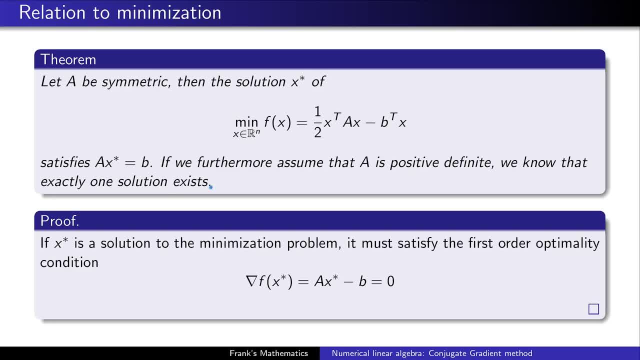 And this is exactly what we want to solve. Okay, if we assume that a is positive, definite, we know that exactly one solution exists. but it is not so important. The main result, The theorem here, is that we can couple our problem with the solution of optimization. 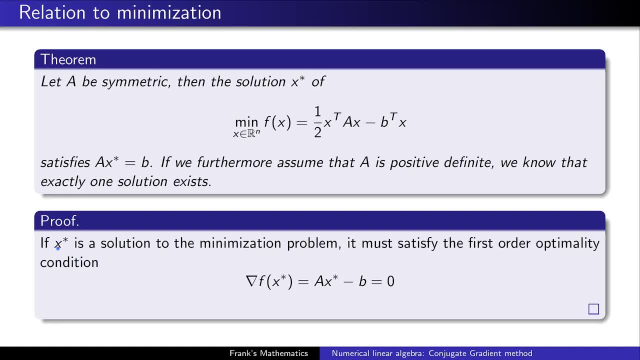 problem. The proof is quite easy. Just assume that x star is a solution to our minimization problem, then of course it must satisfy the first order, optimality conditions. reading the gradient of f must be zero. plug in x star and you end up with a x star minus b. bring b to the other side and you get. 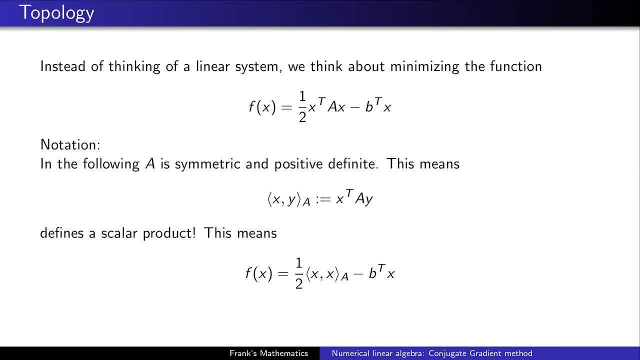 the result of our theorem. Okay, From now on we assume that a is a symmetric and positive matrix. This means that the following function, which contains of two arguments, x and y, which is just x transpose a, y is a scalar product. 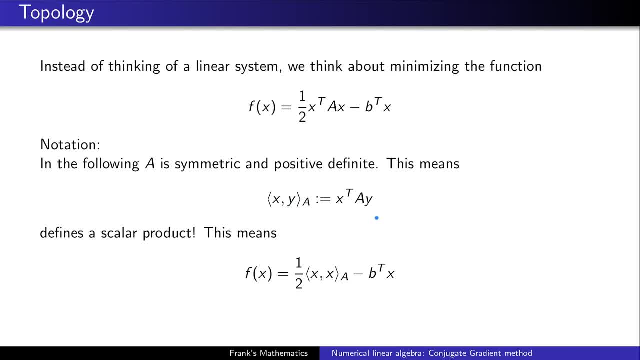 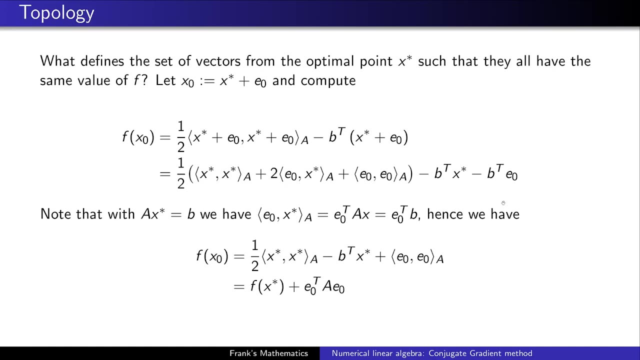 This means it's a bilinear positive definite form. Using this notation, we can rewrite our function f so it just looks like this, And we're going to ask ourselves the following question: What defines f? What defines f? What defines the set of vectors from the optimal point x star, such that they all have the same? 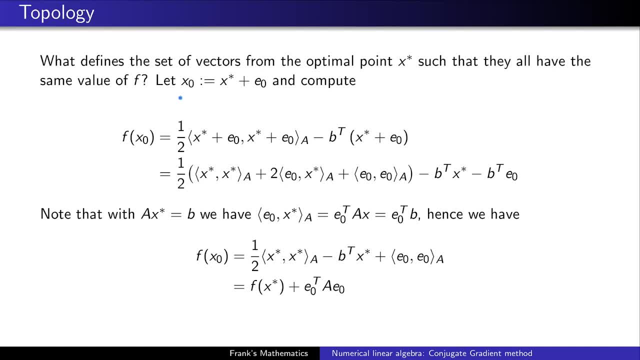 function value of f. To do so we define the vector x zero, which is just x star plus some offset e zero and compute f applied to x zero. Just plug in the definition. you can see it here. Make use that. we have here a scalar product, so it's a bilinear form. split it into the. 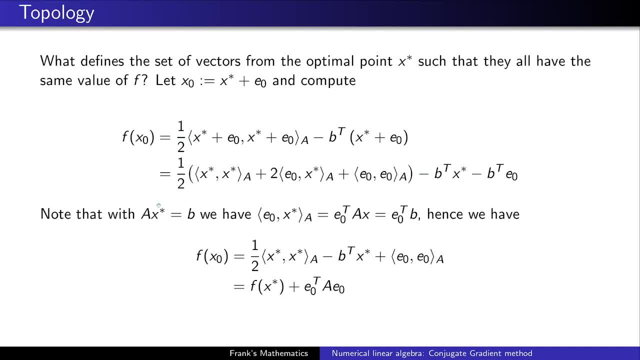 following sets And we end up with this huge long term here. Now we make use that x star is an optimal point of our optimization problem, so this means it satisfies a. x star equals b. This means that we can rewrite our this following term, which is just e zero. transpose a x. 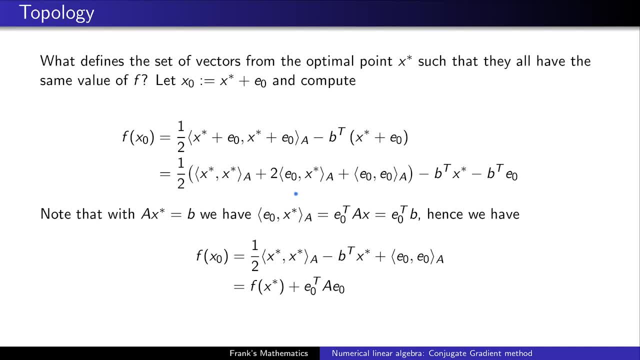 but a, x is just b, So this term here is just e zero transpose b, and it cancels out with this term here. So this term here is just e zero transpose b, and it cancels out with this term here. So basically, we'll end up with the following term: 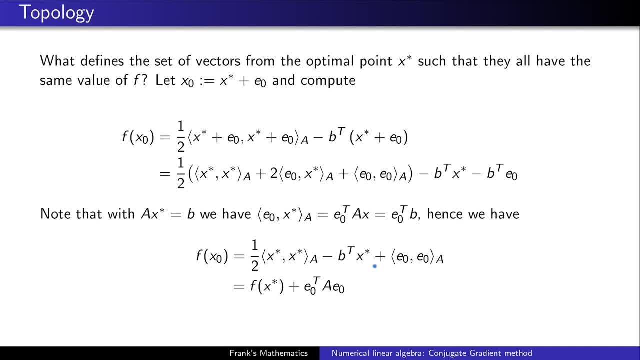 These are the terms that are left, And if you combine these two terms into our function f, it's just, by definition. this is f x, f x star. we end up with f x. zero is just f of x star, which was our optimal. 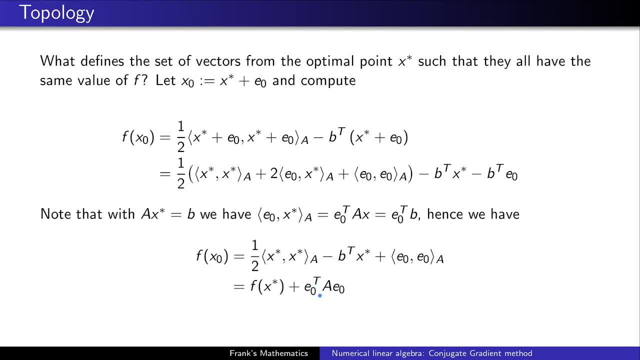 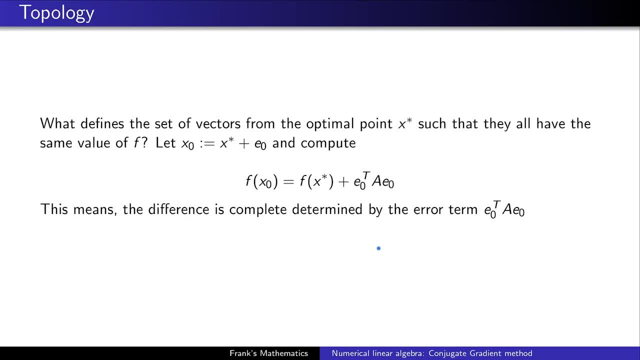 point plus the offset e zero transposed a e zero. This means that the offset of our function f, or in other terms, the difference of x zero and f x star, is completely determined by the following error term, which is just e zero transposed a e zero. 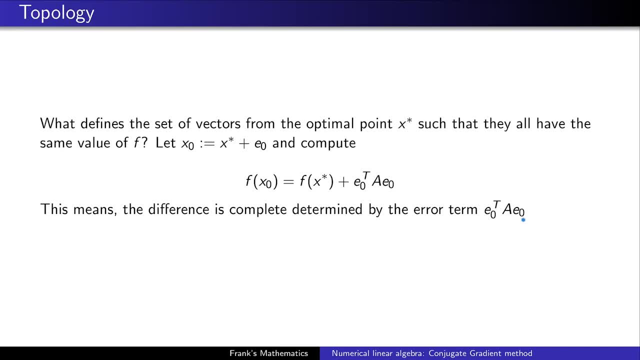 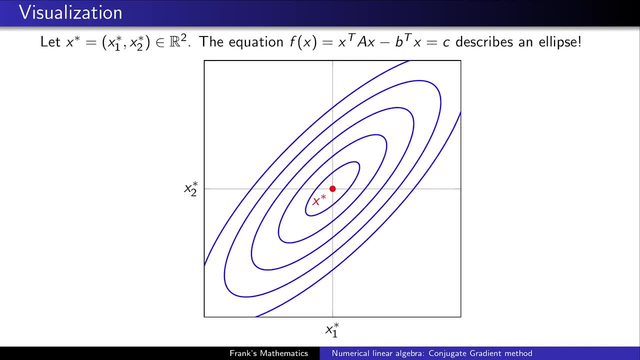 This will come in handy later, because we now can take a look at the structure of e zero transposed a zero. Let's visualize this a little bit Here. we have, you know, two dimensional examples, And our optimal point is now x- one star, and x- two star, which is the component, which the 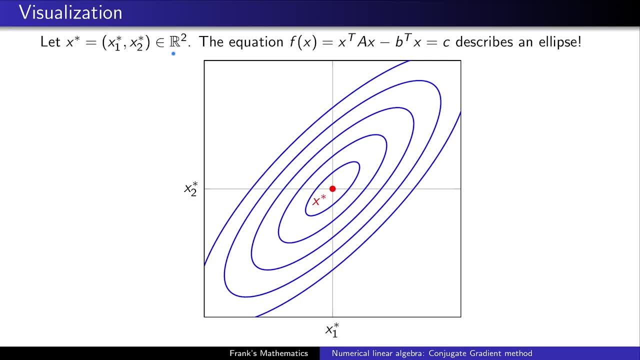 vector in R2.. And we want to take a look at the contour lines, or the lines where our equation, our function f, is constant And this function or this equation f, x, is constant, z. this is describes an ellipse, So you can see the plot here. 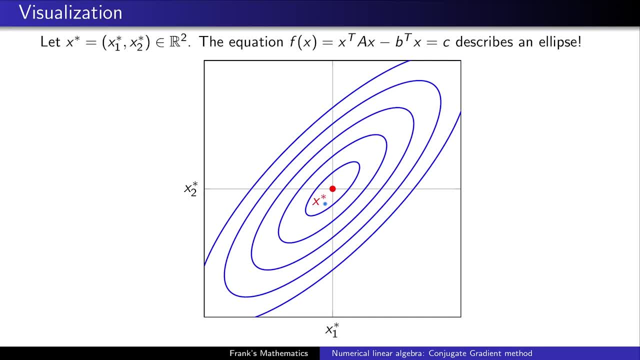 In the middle we have our optimal point, x star, and the blue lines which are circled around x star on. if you travel on this line, the function value of f stays constant. So if I travel here, it's it's it's a constant. if I travel here, it's constant. 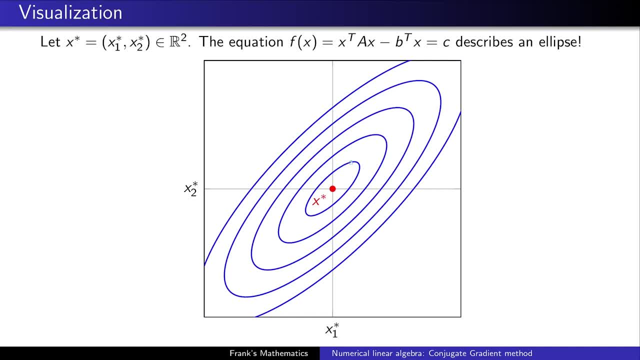 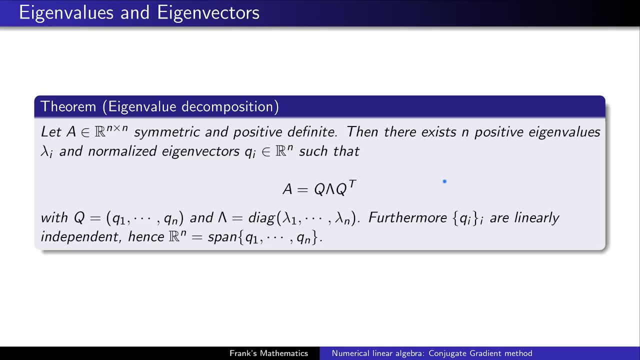 But important thing is the. these blue lines are ellipse, And now we hop in into deep linear algebra, the so called eigenvalue decomposition. we assume that a is symmetric and positive definite. then we know that there exists n positive eigenvalues. they call them lambda i and normalized eigenvectors, which I call q i in the following: 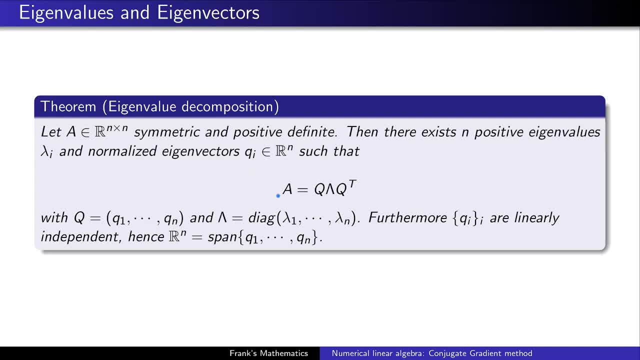 form that we can express our matrix A as the matrix product of q lambda and q transposed. And of course you know that q consists of the eigenvalues. lambda is a diagonal matrix which contains only the, the eigenvalues lambda, lambda i. 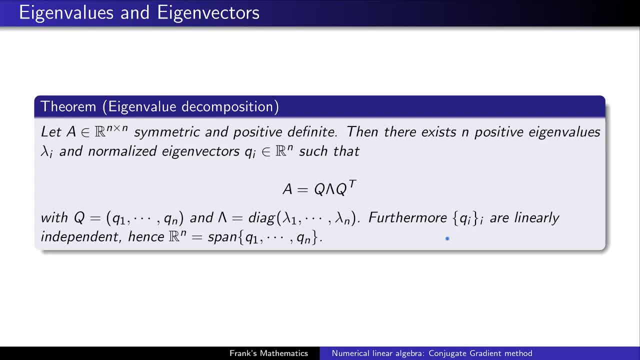 And of course we know, we know, know that q i a linear independent and that inverse of q is q transposed And stuff like that. So this is the classical eigenvalue decomposition And we make use of this, this decomposition, here. 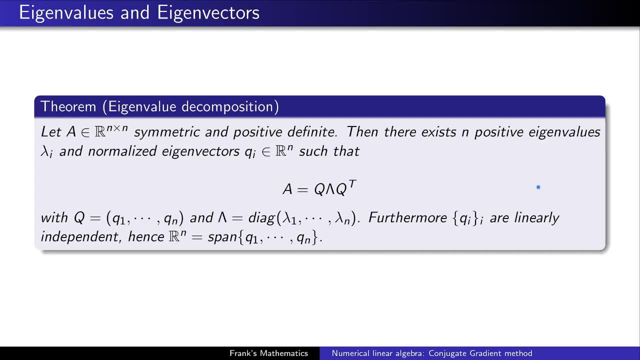 So what we're gonna do now is we're gonna write down the n and q. So we're gonna write down the n and q And then we're gonna write down the n and q space. we define another space, which is the so-called eigenspace. 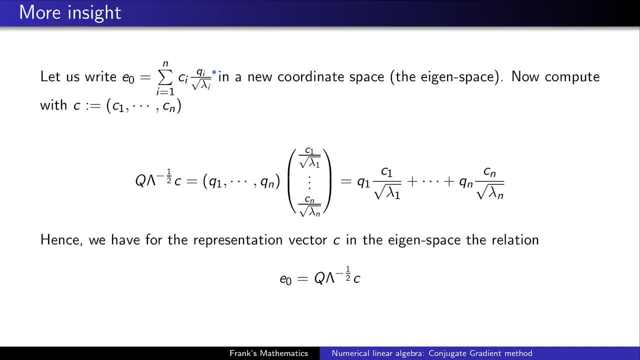 First, we know that qi, which are the eigenvectors, they are linear independent. but this means that qi divided by the square root of lambda i is also an independent set, linear independent set. of course, This allows us to express our offset as a linear combination of our new vectors and 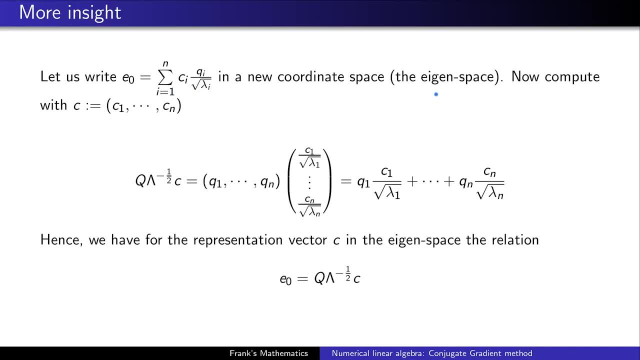 the resulting space I call the so-called eigenspace. And let's do a little bit of calculation. we compute the following expression. First we gather all the coefficients ci, which comes from the linear combination of our expression of e0.. I gather them in vector c. 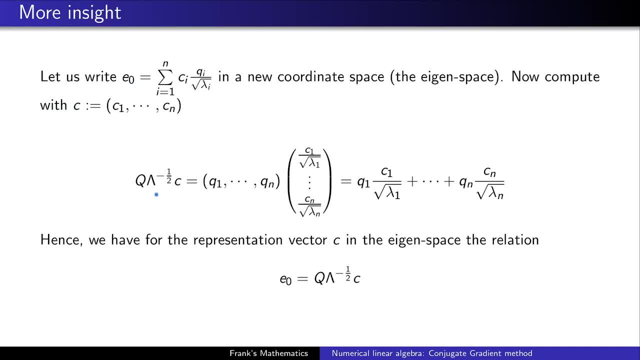 And I calculate q times square root of lambda times c. If you do the calculations here, let's just plot it in here- you can see that this term is exactly e0.. So this means that we have our representation, vector c. We can express them as we have the following relation between our original vector in the: 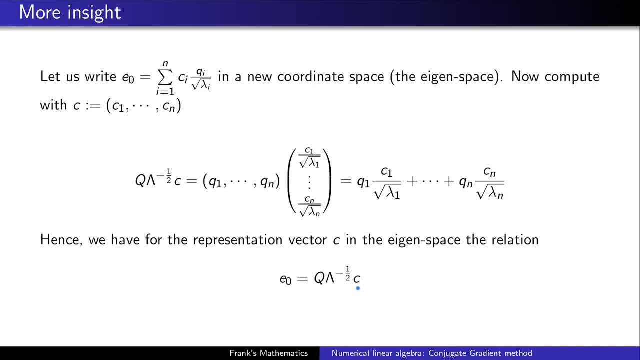 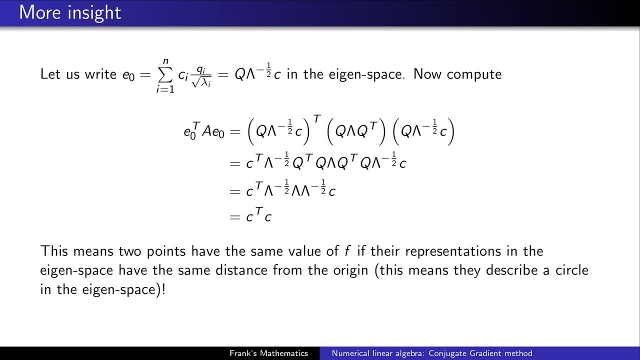 carthaginian space And our vector c in the eigenspace. we have the following relation: e0 is q times square root of lambda times c. We will now make use of this Again. we have: c is the representation vector of e0 in the eigenspace. 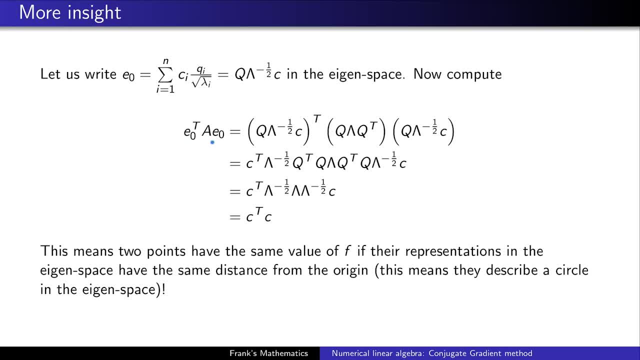 And now we want to compute the following expression: e0 transposed ae0. Because this was the difference between f and f. So this is the term we want to calculate. So take the expression e0 transpose ae0. So this is the term we want to calculate. 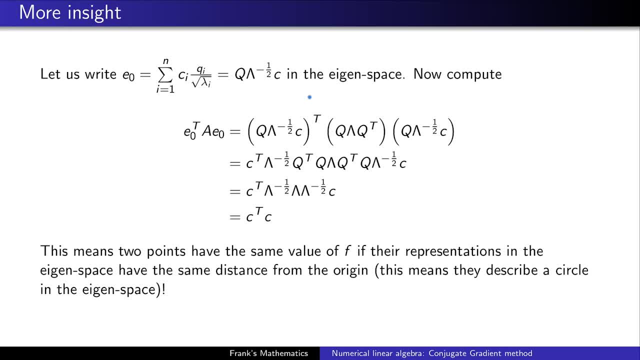 So take the relation e0 and this term here, plug it into this equation, replace a by q lambda, q transpose, And now solve the transpose. So bring it to the other side and what you will end up is the following term: You see, q transpose, q is the identity, so this term drops out. this term drops out. 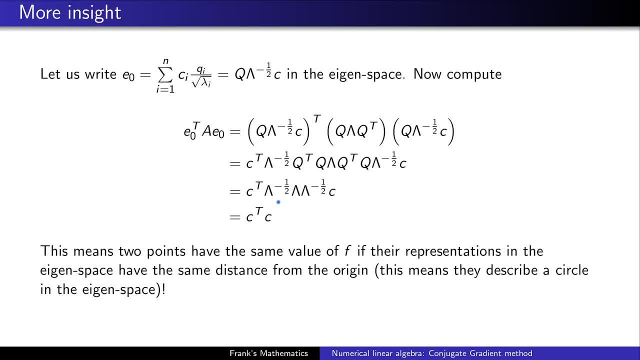 and we end up with the following term: Lavenda times, lamda times. e0- transposeοιπόνat 852. And again, lambda, square root of lambda times, lambda times. square root of lambda is, of course, the identity. So we end up that e0- transpose ae0 is just c- transpose z. 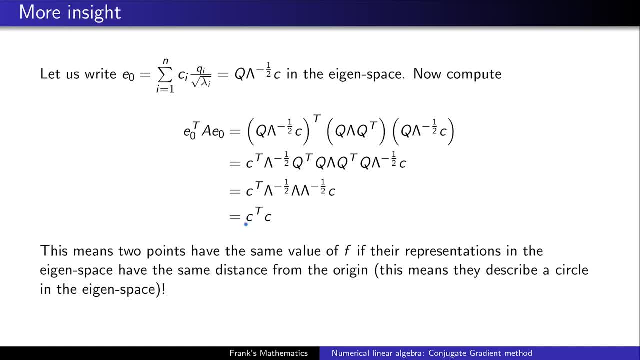 So it sees it's the norm of the representation vector in the eigenspace, computed with the R endpoint norm. So in other terms, Thank you. two points have the same function value if the representation vectors have the same distance from the origin. In other words, they describe a circle in the eigenspace. So remember. 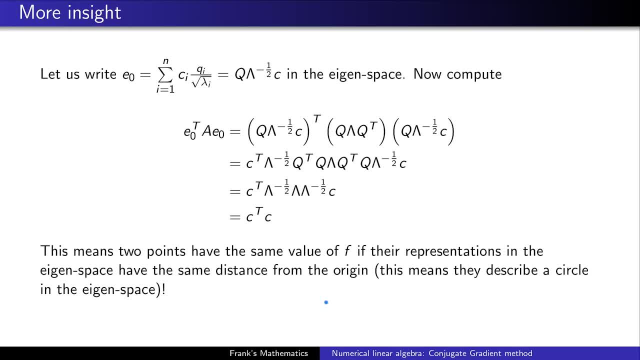 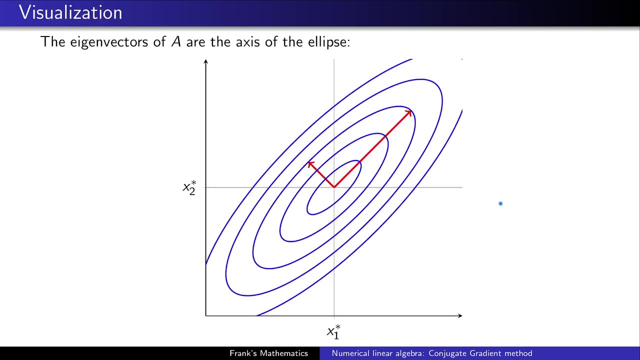 go back two or three slides. the contour lines where f had the same function value describes an ellipse in the standard cathesian space. but they describe a circle inside the eigenspace. So let's have a quick visualization here. Again you have the circles, added ellipses here. 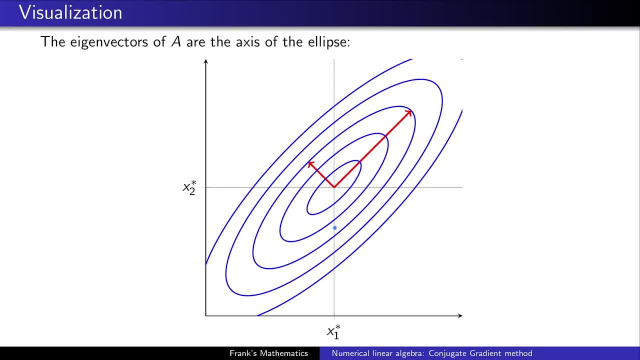 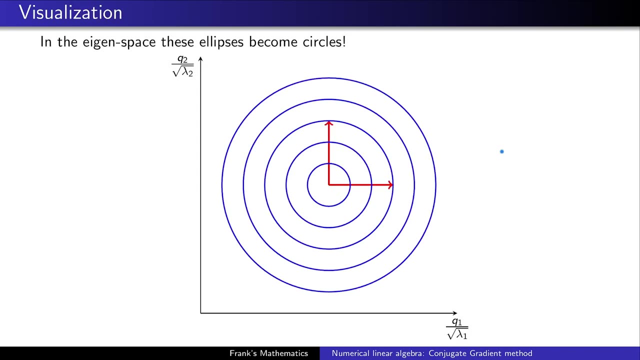 which contains fun, which which contains points with the same function value of f. I draw here the eigenvectors of a, which are of course the axis, the main axis of the ellipse here. And if you transpose the, the, these ellipses, into our eigenspace, well, we end up with circles. So in the eigenspace, 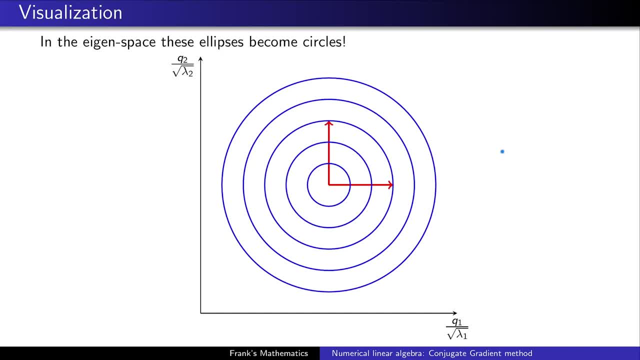 these ellipses, they become circles, And this is, of course, super nice. So this is: keep this in mind, this is, this is what, what's going on with the, with the transformation which we've done so far in the transformation in the eigenspace, And we will make now, of course, 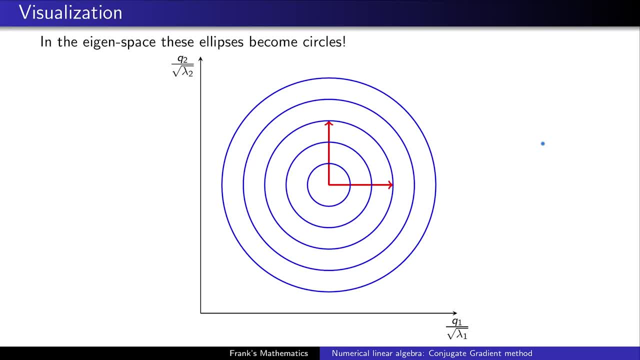 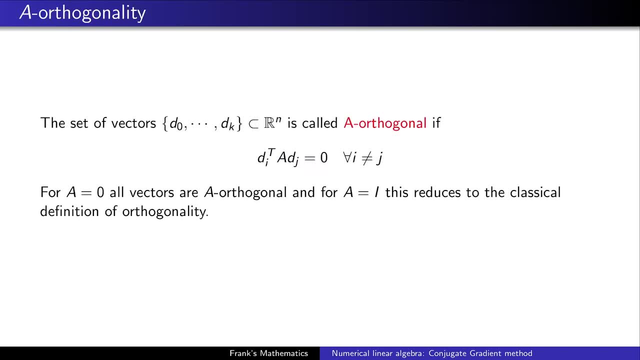 we make heavy use of this. But first we have to put this into into some solid definition. We say that a set of vectors is called a orthogonal if the following condition holds: we compute di, transpose atj, and this must be zero for all i, not equal to j If a is zero. 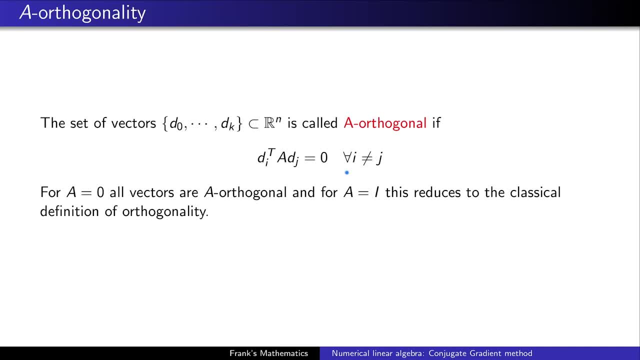 of course all vectors are a orthogonal. this is kind of useless. And if a is choosing to be the identity, this then reduces to the classical definition of orthogonality And this definition is of course the the right definition, definition to care. 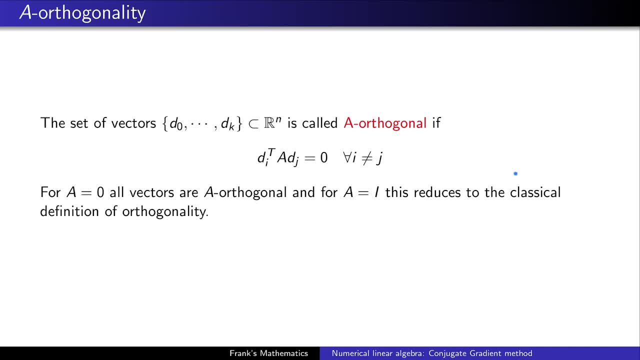 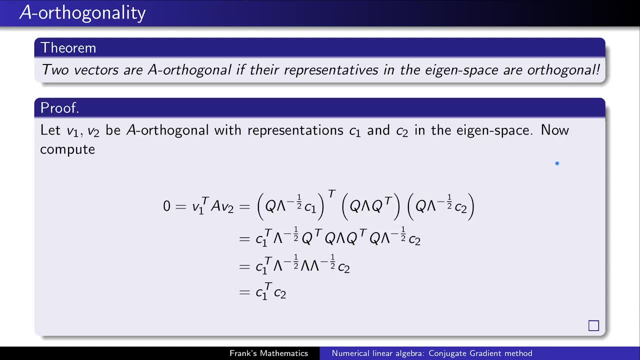 which is to capture orthogonality inside the eigenspace. And this is part of the next, next theorem. Two vectors are a orthogonal if the representatives inside the eigenspace are orthogonal. We assume again that a is symmetric and positive definite. Let's take a look at the 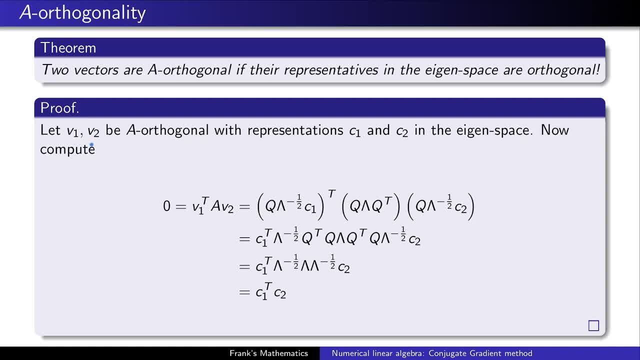 proof. The proof is quite simple. We take two vectors, v1 and v2, they should be a orthogonal- And the representatives inside the eigenspace are called c1 and c2.. I mean now we compute v1, transpose a v2.. This is the same def, the same calculation as 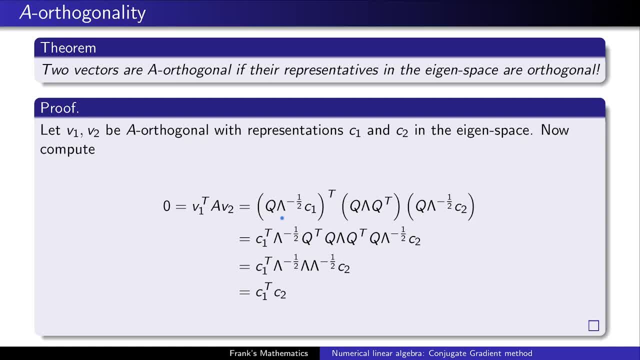 we've done before. we place v1 with q lambda c1, or if q inverse, inverse square root of c1, and similar for v2, calculate those products. those term drops out. this is the identity and we end up this: v1 transpose a v2 is exactly c1 transpose c2.. So this is the correct definition. 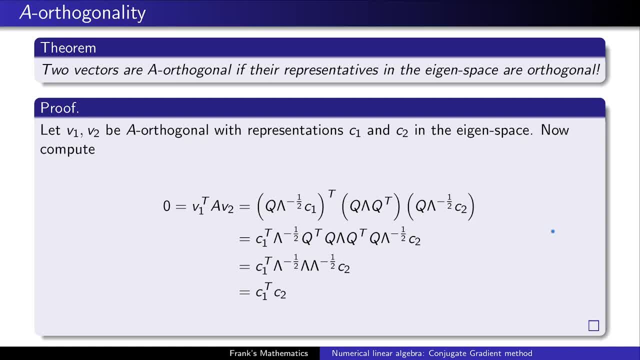 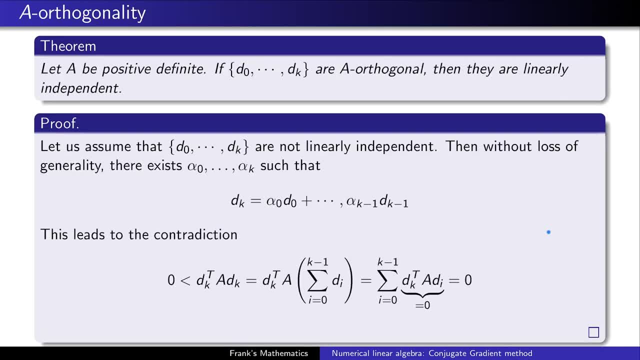 the capture of orthogonality Inside the eigenspace. We know even a little bit more. we know that if we have a set of a orthogonal vectors, then we know that they are linearly independent. The proof is quite simple: is done is done by, by. 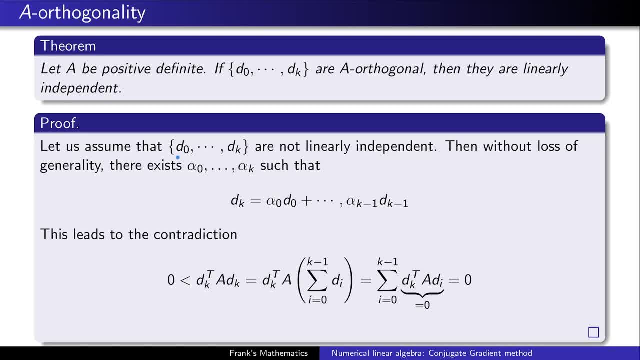 contradiction. Let's assume that the set D zero to decay is not linearly in, is not linearly independent. So we can assume that, of course, without lots of generality, we can express that D? k as linear combination of the zero and up to dk minus one. 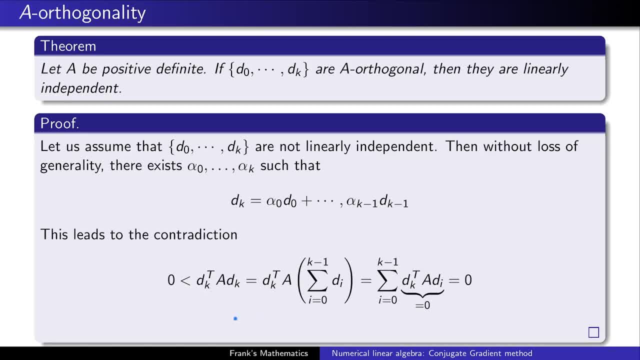 But of course this leads directly to a contradiction because by definition we know that decay transposed, a, D, k is greater than zero. this is a definite definition of the A orthogonality. Let's replace glass decay by linear, linear, linear combination of the zero. 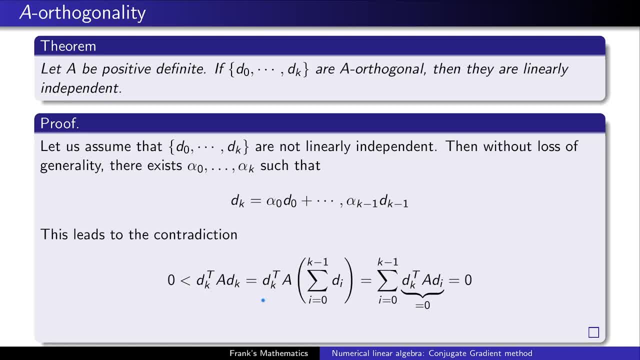 to D, k minus one. you can see it here. put the last, put dk transpose a inside, inside the sum, and you end up with terms containing dk transpose a, d, i, but i is always less than k. so this term again by definition of a, of a orthogonality. 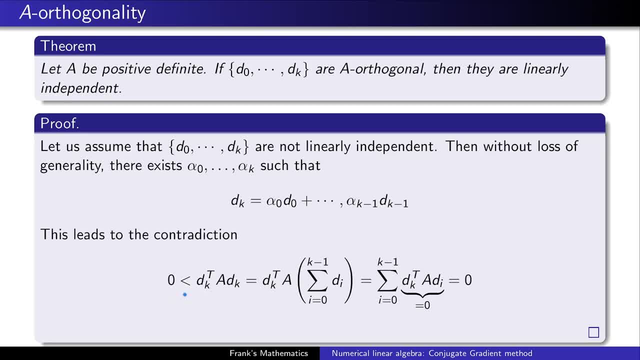 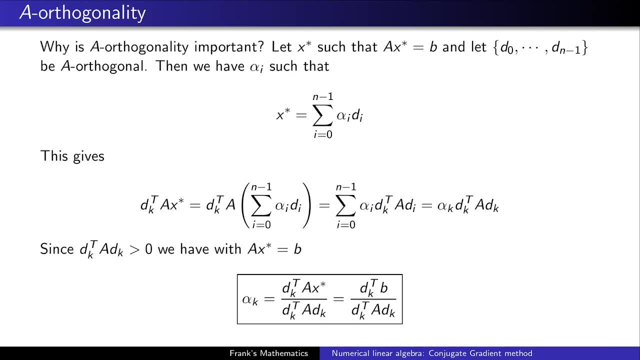 is zero. so this leads to the contradiction: zero is less or strict less than zero. so this proves the theorem. why is a orthogonality useful here? let's assume that x star satisfy a, x star equals b, and let's assume we have a set d 0 to d. 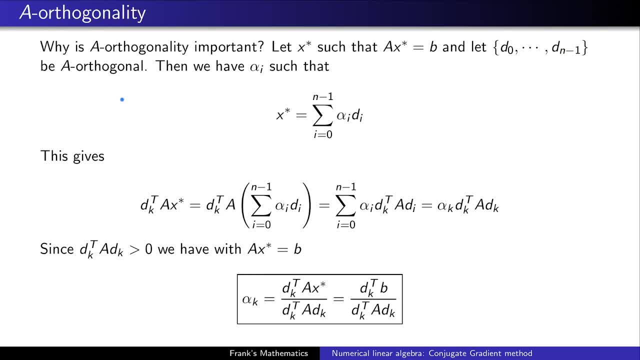 n minus one, which is a orthogonal. by the last theorem, we know that these n vectors are linearly independent, meaning they they form a spanning system, they form a basis, and this means we have a set of alpha i yn in such a way that x-star can be expressed as a linear combination of the d-i. 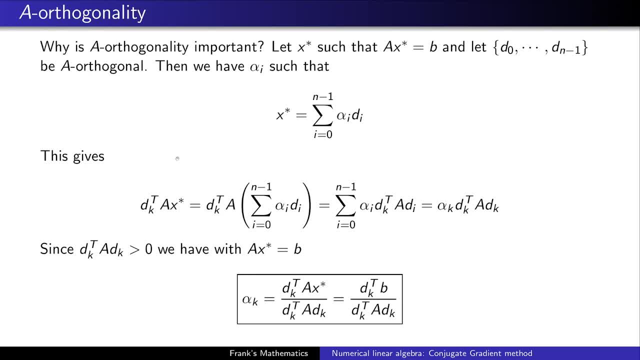 And this is interesting because now we can compute a dk-transposed, a x-star. Let's replace x-star by the linear combination of the d-i. you can see it here Again. move dk-transposed inside the sum and you will end up with terms containing dk-transposed. 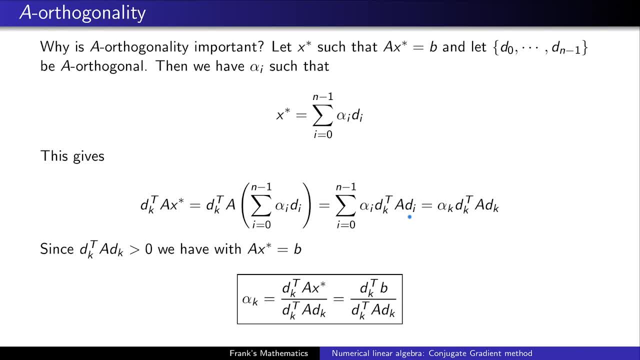 a d-i. And this is perfect because by a-orthogonality we know this is zero, except if a is equal to k. So this means: dk-transposed a x-star is alpha k. dk-transposed a dk. We know a little bit more, we know this term. dk-transposed a dk is greater than zero. 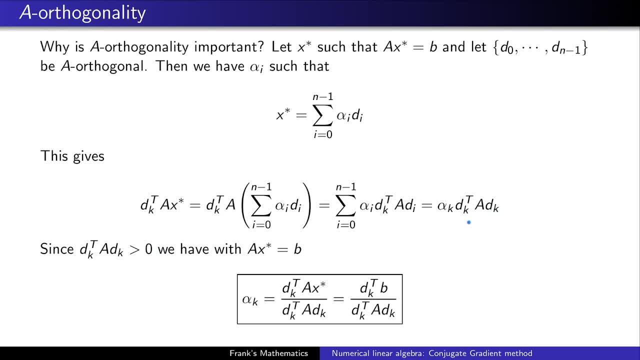 So let's divide this expression by dk-transposed a dk And we end up with a dk-transposed a x-star. So we have alpha k being dk-transposed a x-star, divided by this term. here We have not used yet that a x-star is b. 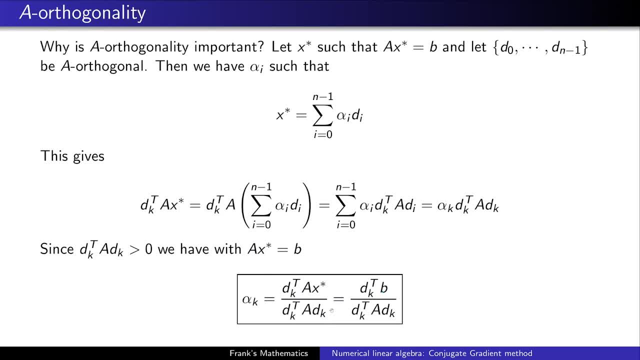 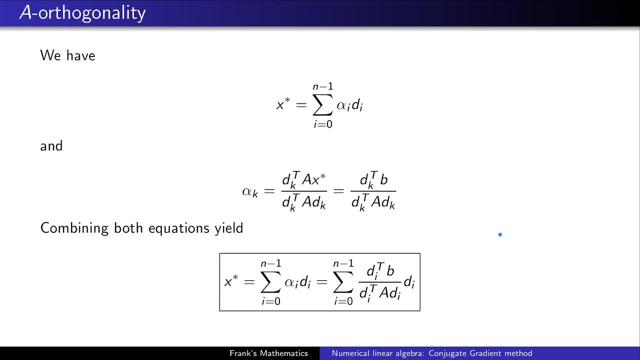 So let's replace a x-star with b, And we know that alpha k is the expression you can see here on the right hand side. Why is this good? why is this useful? You can see again here x-star as a combination of the d-i. here you can see our calculated. 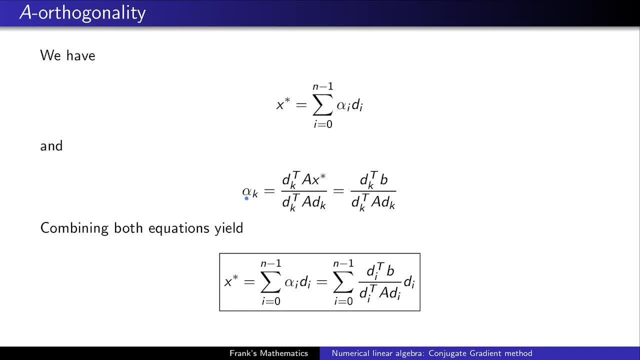 expression for alpha k. Okay, So let's put everything together. We know x-star is linear combination and we know alpha i, So let's replace alpha i by our result we just obtained, And you end up that x-star is the sum of this term here. 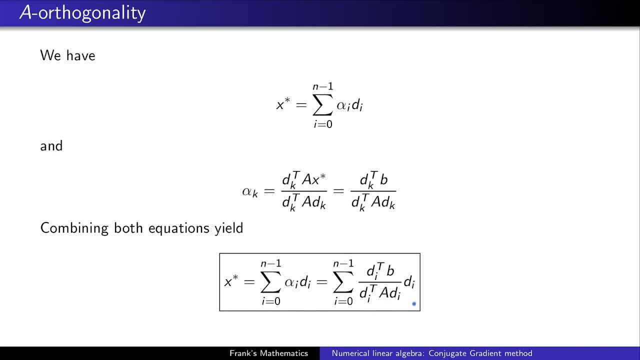 It might look a little bit complicated, But I want to point out something. It is very interesting that we do not see x-star on the right hand side. We only see A and B. but A and B are known. We know this a priori. 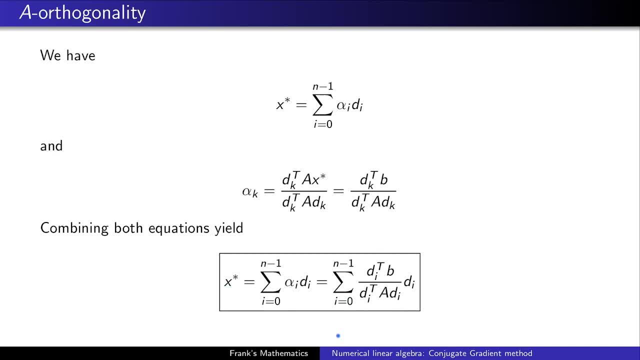 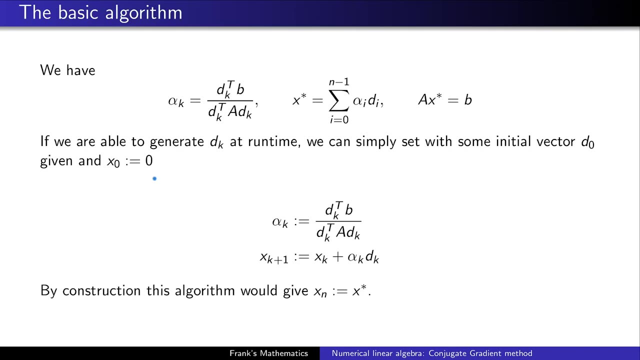 What we didn't know a priori is X star, because we want to compute X star. So this is interesting because this gives us the possibility to form or to formulate a very basic method. Again, these are the same terms I just presented to you. 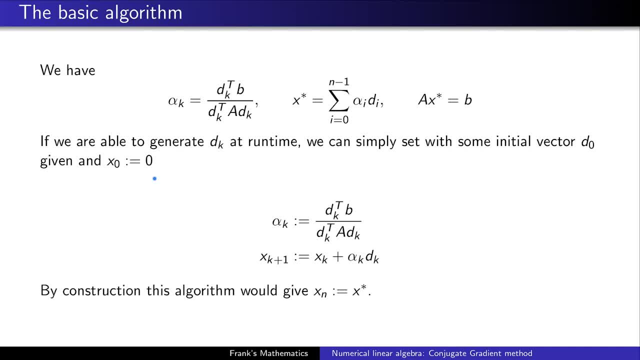 Because if we are able to generate an A orthogonal set, we can simply compute these alpha Ks and compute X star. because we know then, alpha I, Alpha I can be computed, knowing only the matrix A and B. And well, just compute a linear combination and you are done. 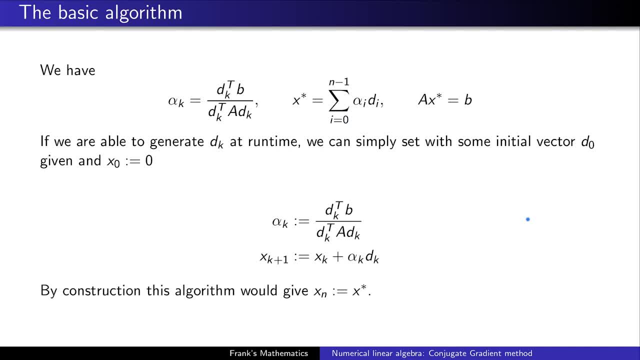 And this is the very basic algorithm of the conjugate credit method. Okay, Let's take a look at a bit in detail. We start with X zero being zero And of course we can calculate X K plus one is X K plus alpha K DK. 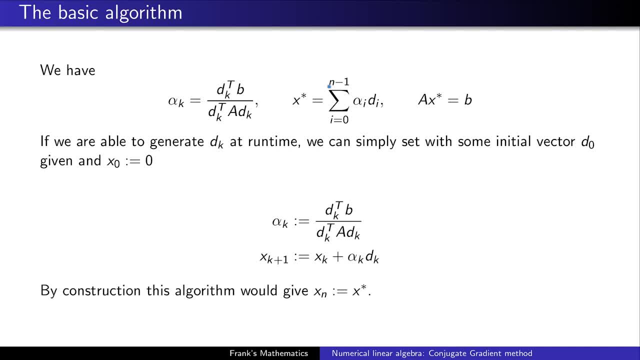 If K plus one is N, we end up with this linear combination of the DIs, which is, of course, by construction, X, X, star. So all we have to do now is to find a method how we could generate those A orthogonal vectors at runtime. 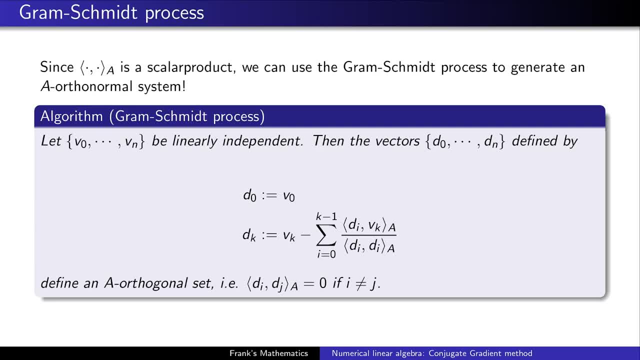 Now it comes in hand that we have a scalar product defined at the very beginning of the video because, if you remember, X transpose A Y, which was our scalar product defined by subscript A. we can use the standard Gram-Schmidt algorithm to generate an A orthogonal system because, by definition, the Gram-Schmidt algorithm generates a sequence which is orthogonal with respect to the A orthogonal system. 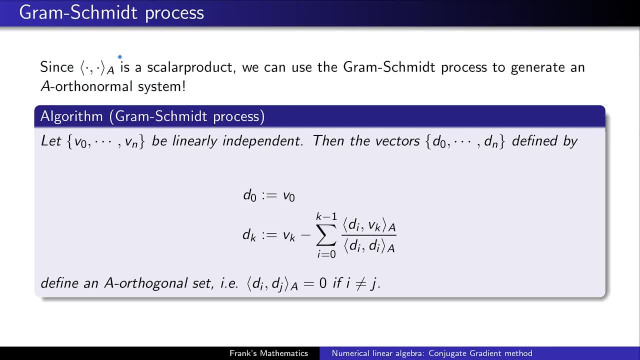 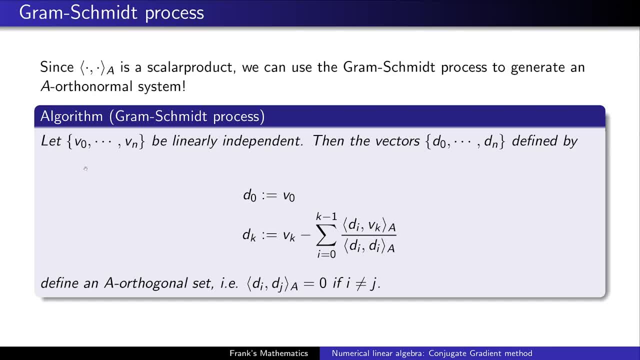 Okay, Transcendent, here is less safety. to integrate this then to the other one Okay set of vectors which are called v0, and these vectors will be used to generate a set of vectors d, which are an a-orthogonal set of vectors, and it is just done simply by subtracting the 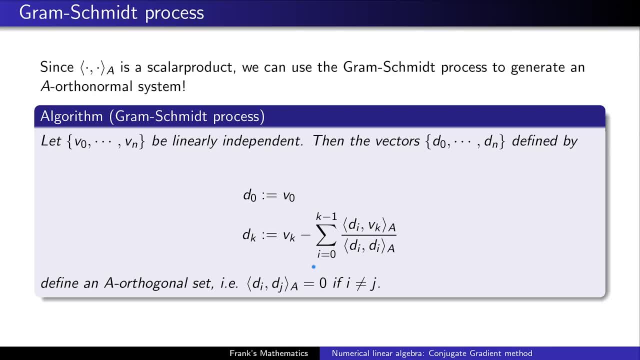 non-orthogonal part. This is a very basic idea of the Gram-Schmidt process. again, I'm not going into details here, but at the end we will end up with an a-orthogonal set, and this is perfect, because this is all we are left in our conjugate graded method, our very basis, just one slide before. 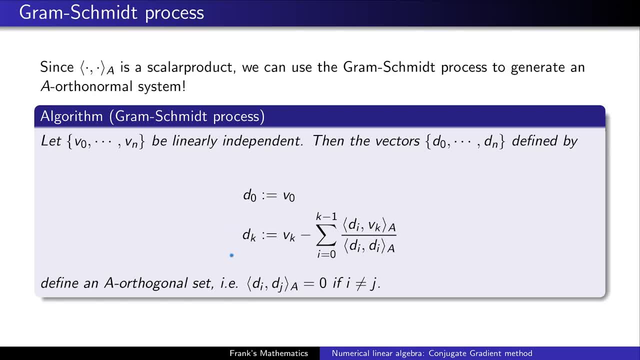 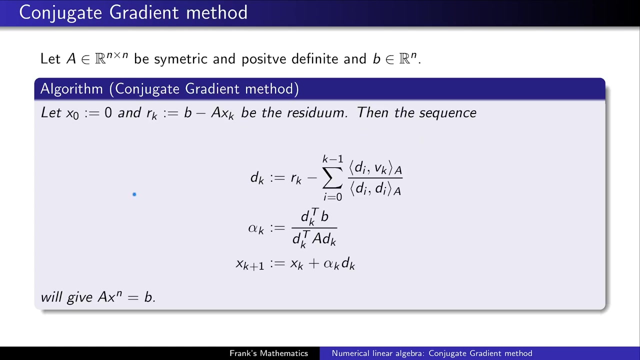 So let's take the definition of the or the outcome of the Gram-Schmidt process and put it into our conjugate graded method. Just one detail: the Gram-Schmidt process needs some sort of independent vectors to generate an output, and we will choose this to be the residuum. So again, we assume a to be a symmetric. 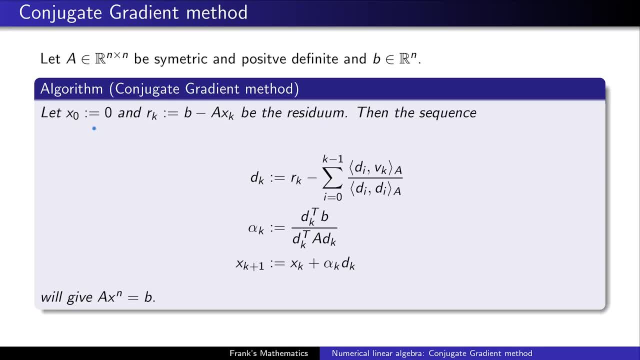 and positive definite matrix. We start with x0 being zero and now we define the residuum, which is just b minus axk, and we call this rk and we use Gram-Schmidt to generate an a-orthogonal system using the residuum. You can see this here. this is the outcome of the Gram-Schmidt algorithm. 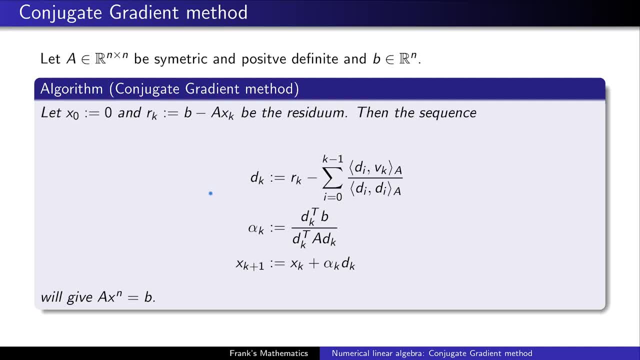 You can also use the Gram-Schmidt algorithm. if you apply the algorithm to the residuum, Alpha k again are the calculated coefficients of our linear combination of x star. and this is just iterative process to generate x star At the end by construction. this will give. 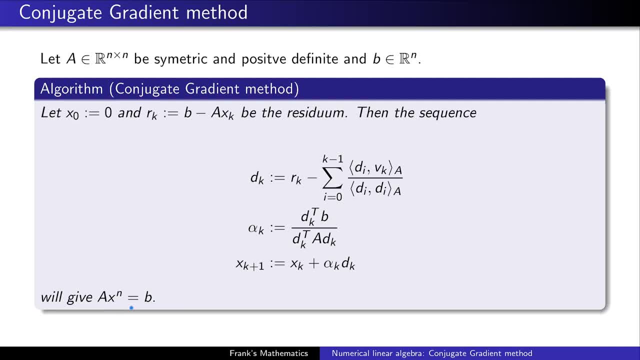 axn to be b, and this is nice. this is the conjugate graded method in all its beauty, Because these are just three lines here, but in these three lines we have to put a lot of theory inside. I mean, we started with moving some vectors and some ellipses to the eigenspace. 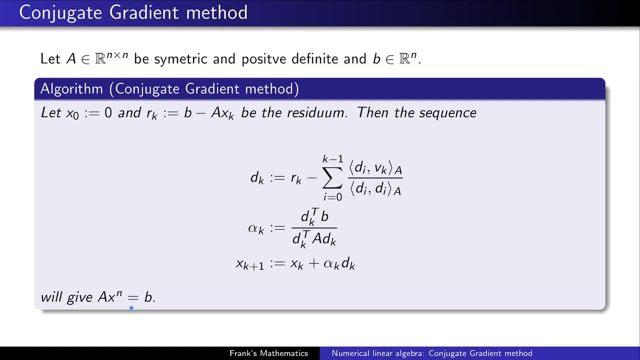 You have to define what does mean. what is orthogonality inside the eigenspace? How does this transform back to the Euclidean space, to the standard space? And there's a lot of theory going behind it, But in the end you have a method which will generate the exact solution after n steps. 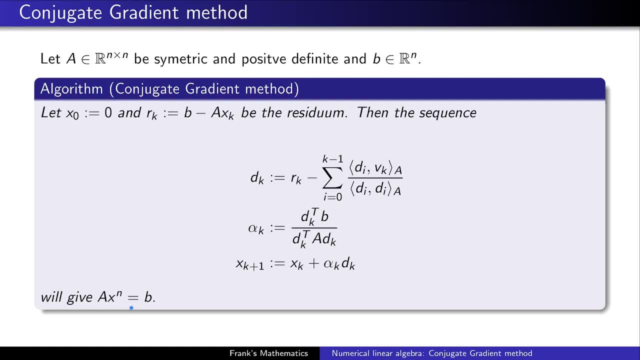 And this is interesting because the standard algorithms, they, only give an approximation, but this algorithm will give the exact solution after n steps. Of course we do not consider numerical errors here, But this is the very idea of the conjugate gradient method. 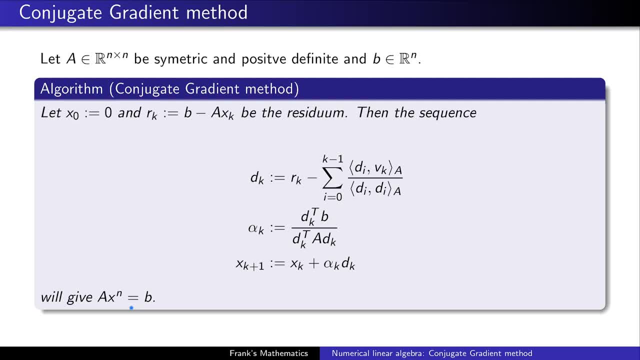 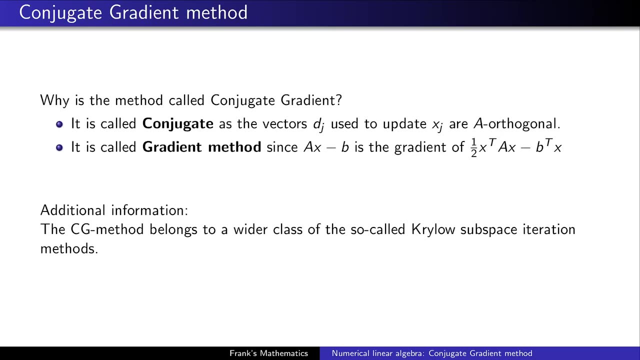 So just generate an a orthogonal set of vectors And use our theory to generate a linear combination of these a orthogonal vectors, which in the end, will give us the exact solution of our system. So there's one last question we have to answer: Why is this method called conjugate gradient method? 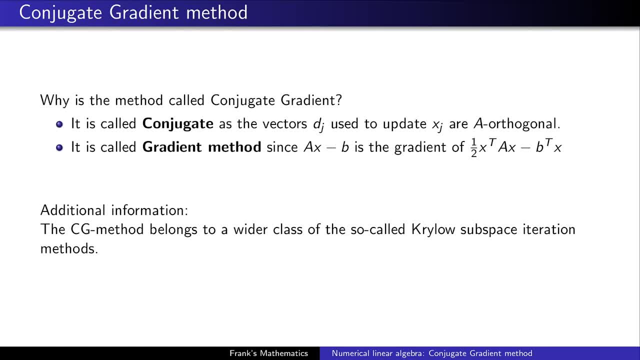 Well, it's called conjugate because the vectors dj, which are used to update the iterates x, xj, they are a orthogonal. So we have a set of vectors, We have a set of vectors. We have a set of vectors.